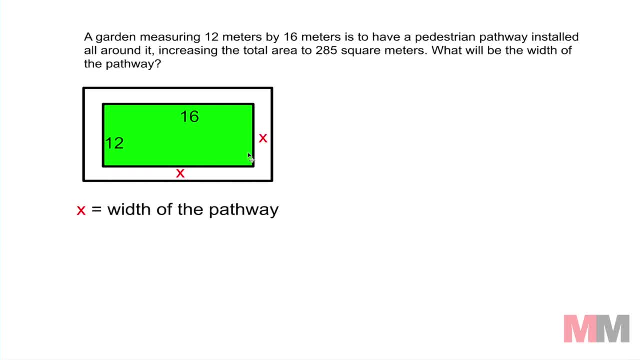 We're trying to find the width and we're just going to call that x of this pathway, So x represents the width of the pathway. They also give us another important information right here, saying that the overall area is 285 square meters, Seeing that this is a rectangle. to find the area of a rectangle you just do length times. 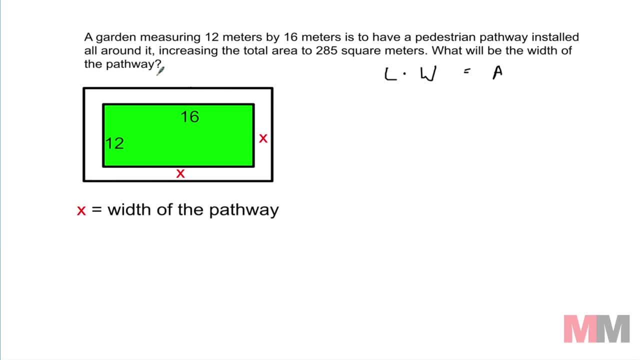 width to get the area. So I first need to find the total length of this overall rectangle. and the length is right here. If you really observe the length, it's made out of this 12 and two pieces of x, because this is x long, x meters long. 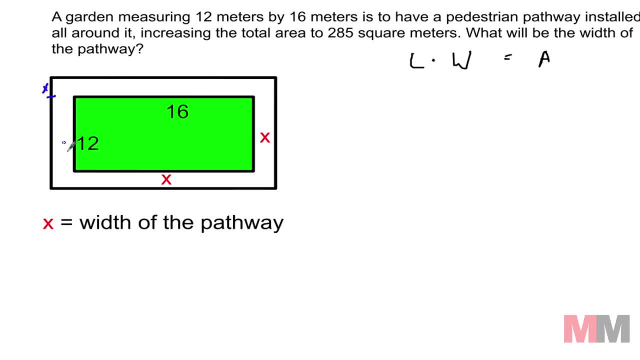 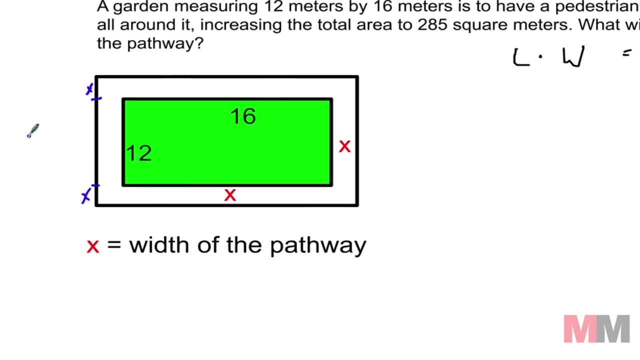 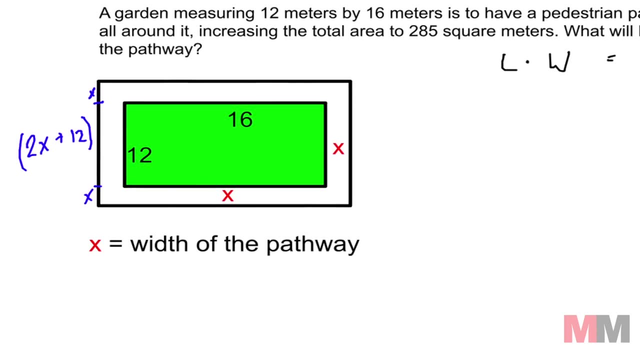 So if I know that that's x meters long and the bottom is also x meters long and this is 12, then I can call this total length 2x, 2x coming from these two x's plus 12.. So we're going to put that in parentheses like that: 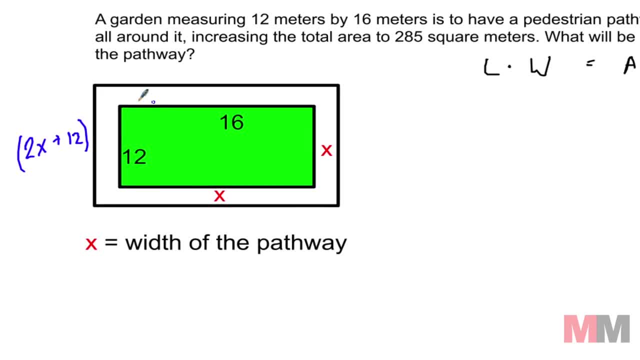 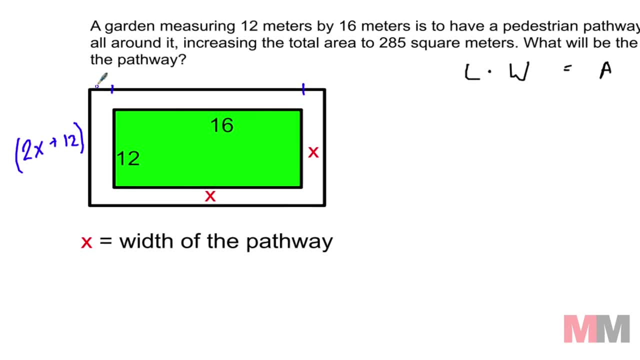 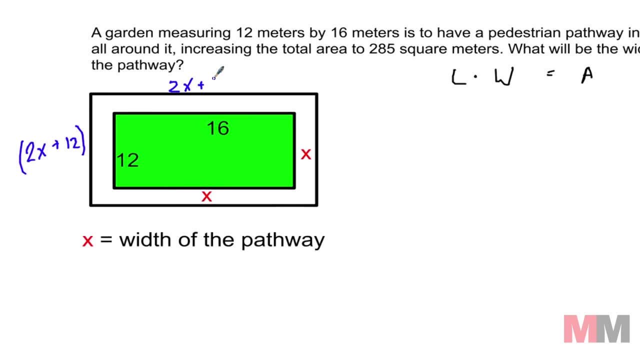 The same logic can be done to find the width. So this is 16 and, as you can see, two pieces with the 16, two pieces of x. with this, 16 makes up the total width: 2x plus 16.. Okay. 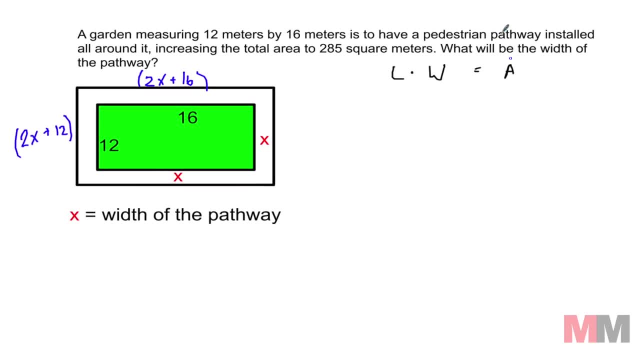 Now that you have a length and width and we also have an area, all we have to do is substitute our length and width with this area formula. So what is my length? So we just said that that was 2x plus 12.. 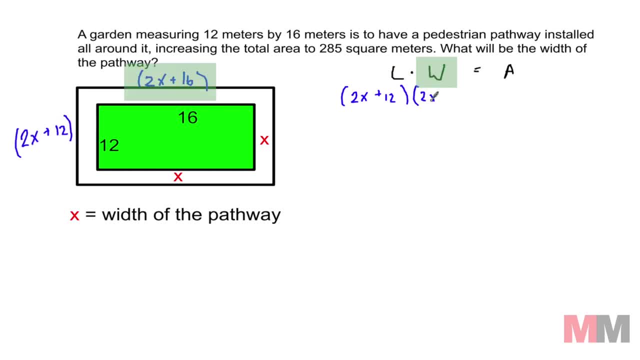 And what is my width? We just said that that was 2x plus 16 equals my area. My area is 285.. If you take a look at what you just wrote, it's an equation for x, And once you solve for x, then we have solved the word problem. 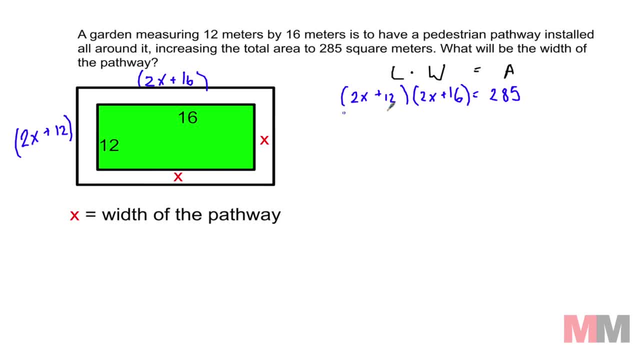 So first thing you're going to want to do, if you look at that, is if you were thinking distribute, then you are correct. Just distribute out these binomials 2x times 2x, That is, 4x squared 2x times 16 is a positive 32x, 12 times 2x. I like to write it under this when they're: 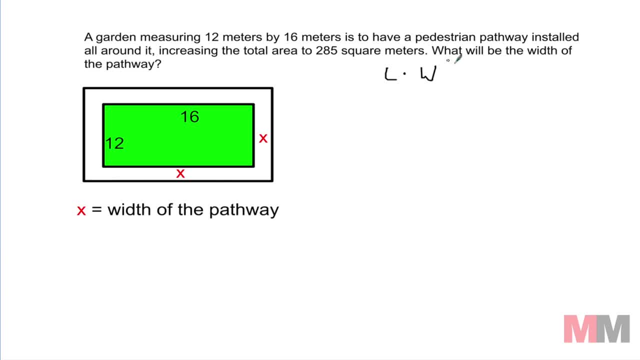 a rectangle. you just do length times width to get the area. So I first need to find the area of a rectangle. You just do length times width to get the area. So I first need to find the total length of this overall rectangle. and the length is right here, If you really observe. 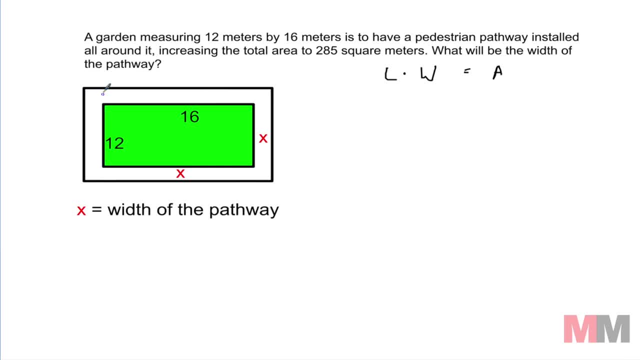 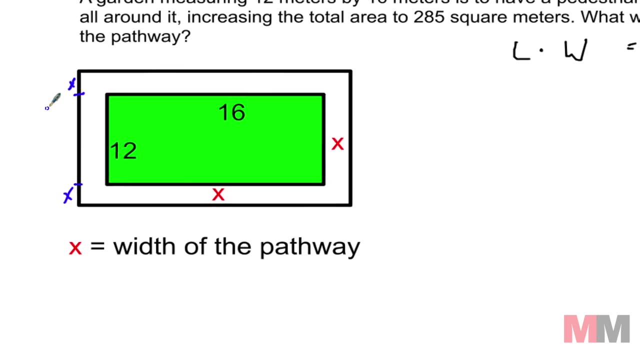 the length it's made out of this 12 and two pieces of x, because this is x meters long. So if I know that that's x meters long and the bottom is also x meters long and this is 12, then I can call this total length 2x coming from x and 2x. 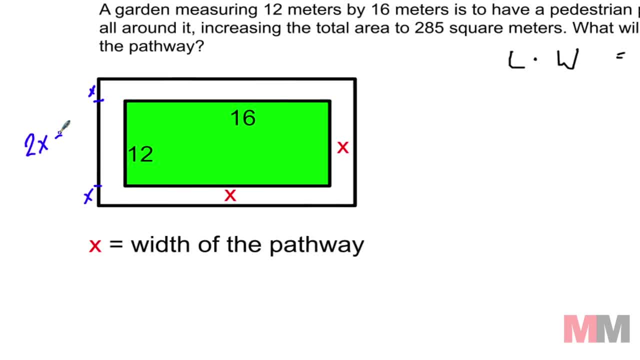 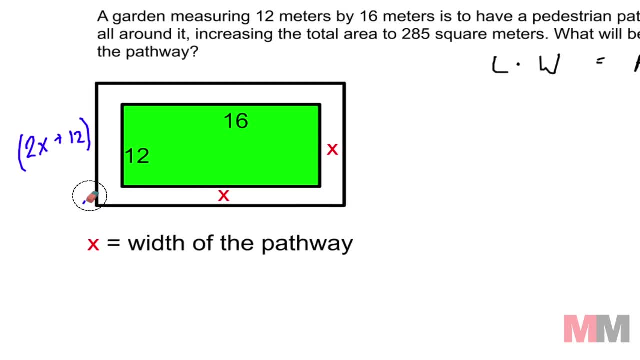 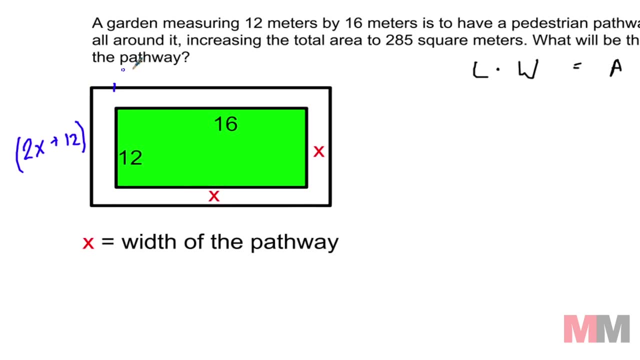 2x coming from these two x's plus 12.. So we're gonna put that in parentheses. like that, The same logic can be done to find the width. So this is 16, and, as you can see, two pieces with the 16,. 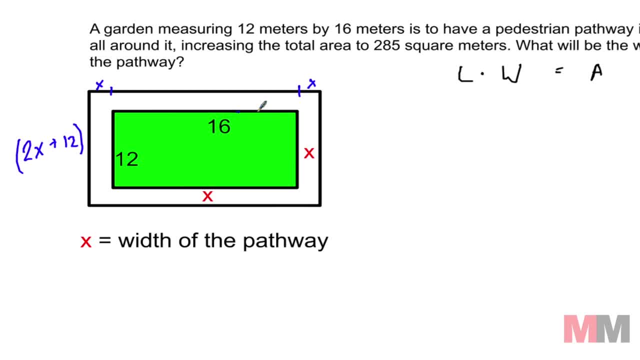 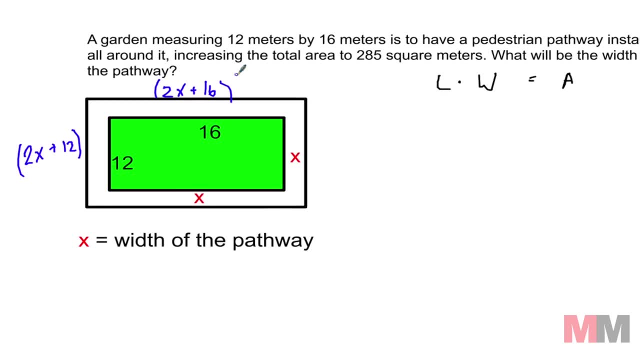 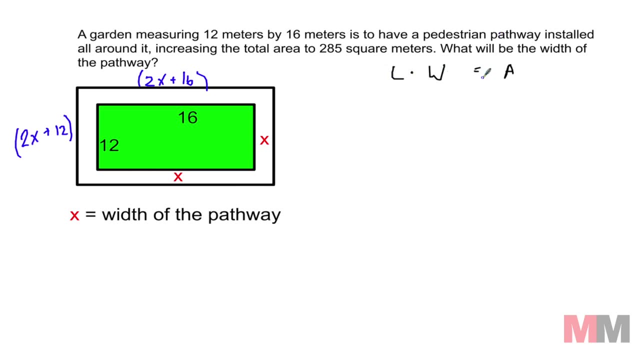 two pieces of x. with this, 16 makes up the total width, 2x plus 16.. Now that you have a length and width and we also have an area, all we have to do is substitute our length and width with this area formula. 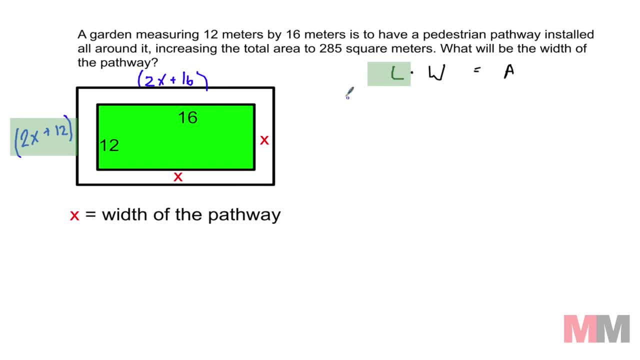 So what is my length? So we just said that that was 2x plus 12.. And what is my width? We just said that that was 2x plus 16 equals my area. My area is 285.. If you take a look at, 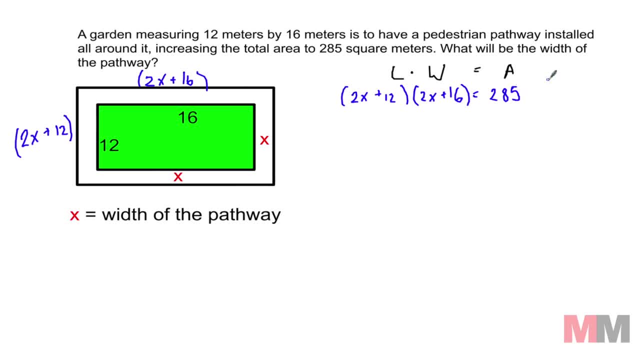 what you just wrote. it's an equation for x, And once you solve for x, then we have solved the word problem. So first thing you're gonna want to do, if you look at that, is: if you were thinking distribute, then you are correct. 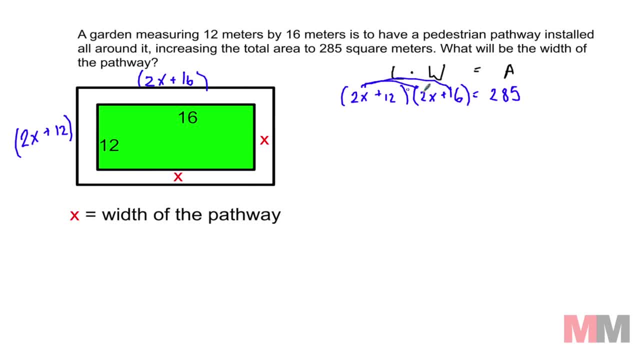 Just distribute out these binomials: 2x times 2x, that is, 4x squared, 2x times 16, is a positive 32x, 12 times 2x. I like to write it under this when they're like terms: